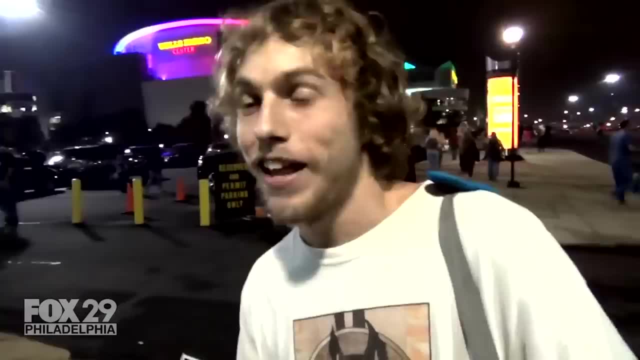 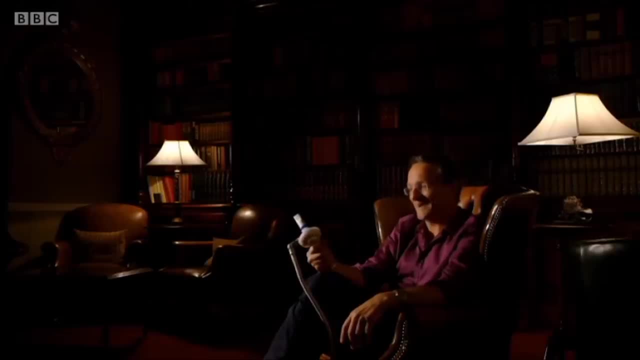 Nitrous oxide has become an ever-increasing worry. A lot of people really love nitrous oxide- Nitrous oxide, aka laughing gas, And it's no laughing matter. I can see why they call it: laughing gas Makes you laugh. They want to suck on them balloons, but everybody fucking sucks at. 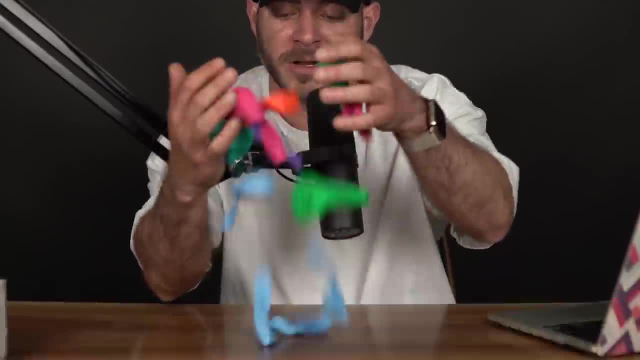 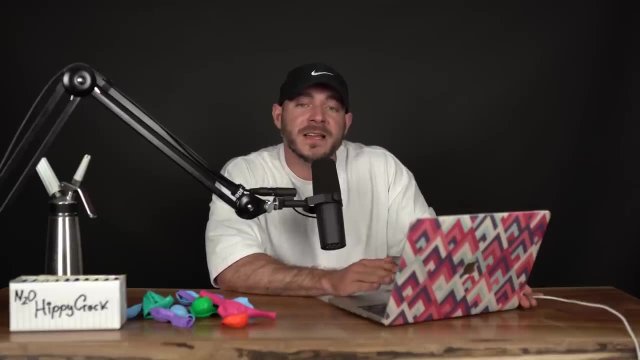 them. First of all, let's start off by explaining what laughing gas is. What are balloons? I mean not these actual balloons, but this stuff. Now, before we do explain, I need to make it crystal clear that I am making this video for safety and harm reduction. Whippets are completely legal. 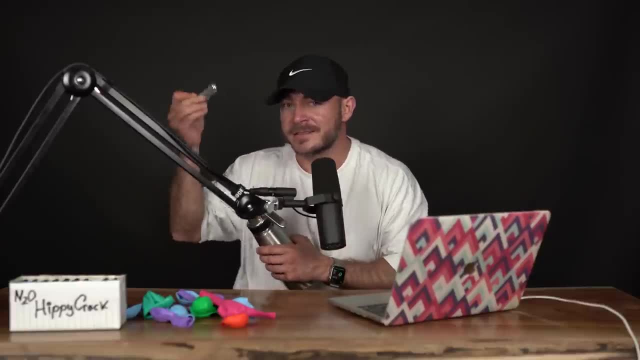 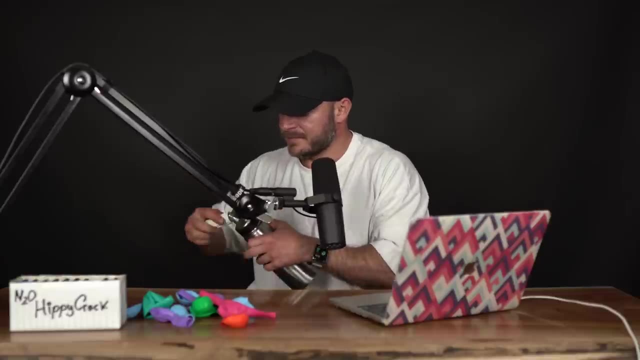 in fact, this is a whipped cream maker. So what you do is you take one of these, throw it in the top here and then you would mix your cream in the base of this and you get whipped cream. But people discovered that not only, it gives you like a very interesting kind. 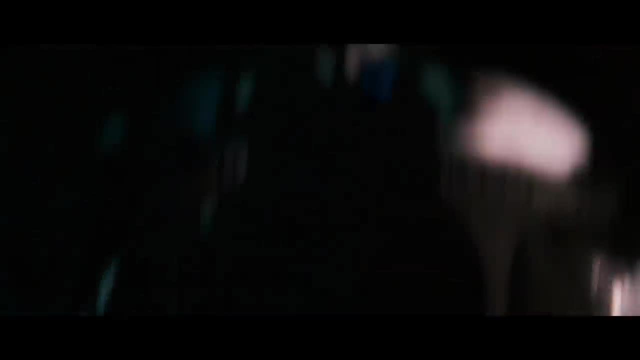 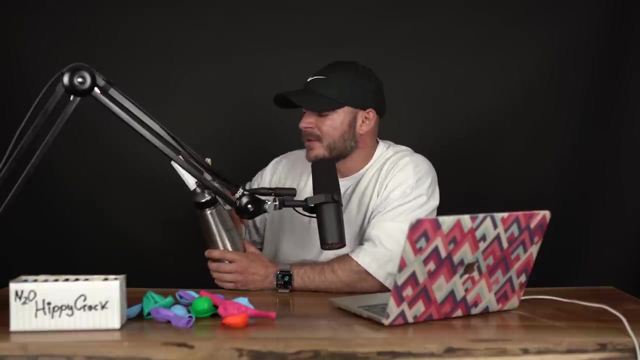 of high, but it also speeds up your car. I need NOS. That's the same stuff. That is this stuff. So yeah, cream goes in here, nitrous in here, and then you squeeze this Cream in there. cream comes out. Right now, it's just. 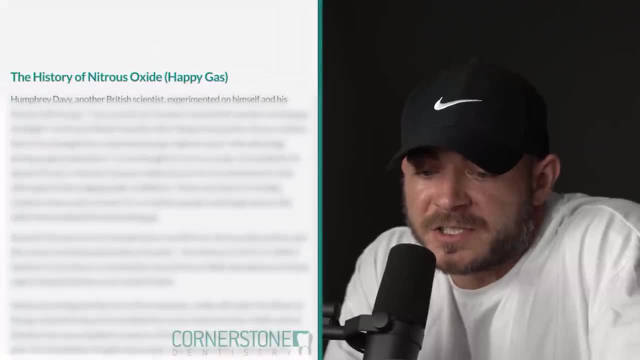 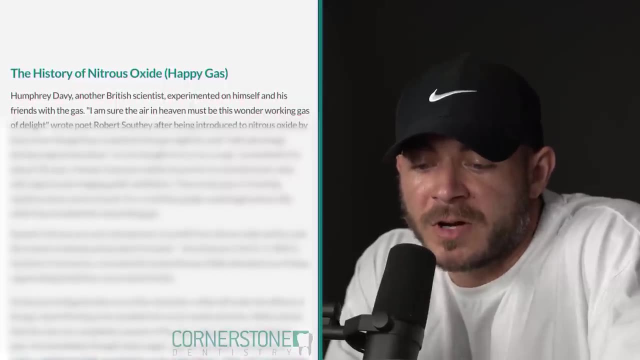 So let's read about the history of nitrous oxide. Humphrey Davy, another British scientist, experimented on himself and his friends with the gas. I am sure the air in heaven must be this wonder-working gas of delight, wrote poet Robert Southey after being introduced to nitrous oxide. 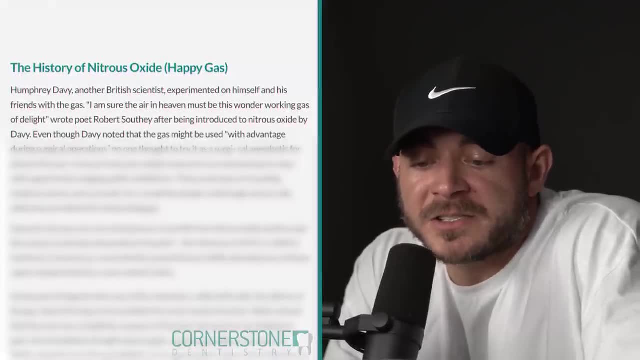 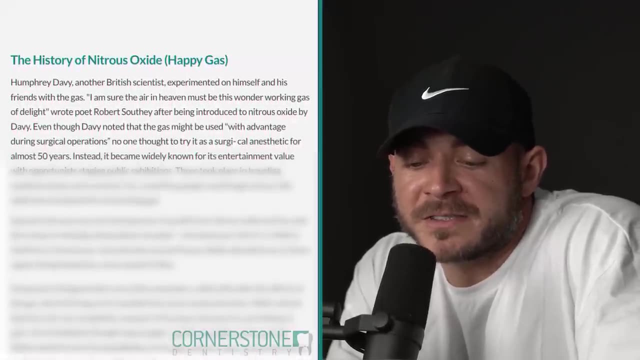 by Davy. Even though Davy noted that the gas might be used with advantage during surgical operations, no one thought to try it as a surgical anesthetic for almost 50 years. Instead, it became widely known for its entertainment value, with opportunists staging public exhibitions. These 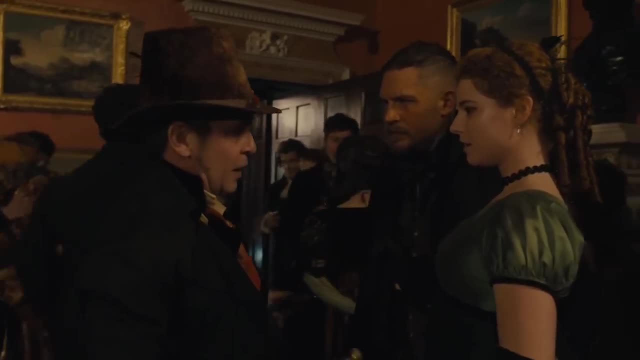 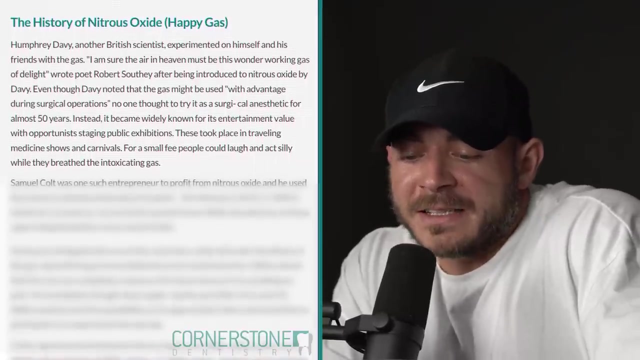 and traveling, medicine shows and carnivals. They call it laughing gas. I provided for entertainment in society parties. It's good money For a small fee. people could laugh and act silly when they breathe the intoxicating gas. Samuel Colt was one of such. entrepreneur to profit from nitrous oxide and use the money to develop and 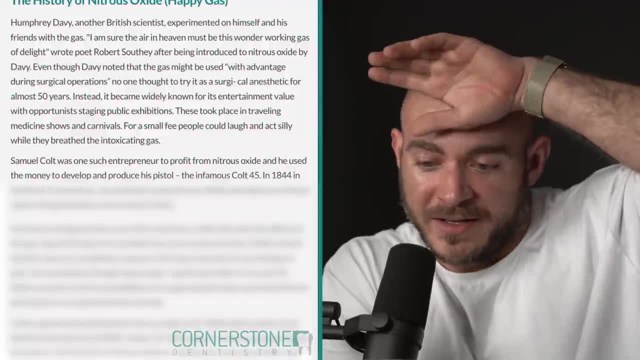 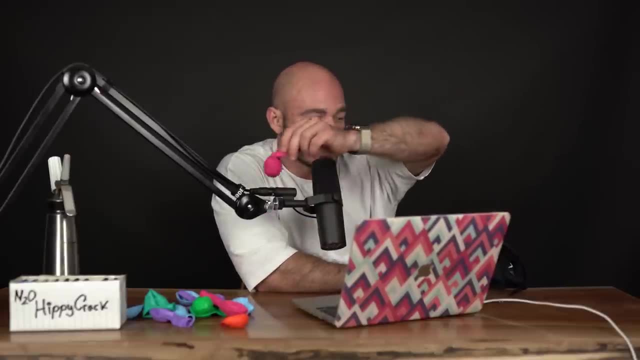 produce his pistol. the infamous Colt 45.. Oh wow, I had no idea. So there you go, the history of the infamous Colt 45. He made money from laughing gas. Laughing gas to guns, That's crazy. He became 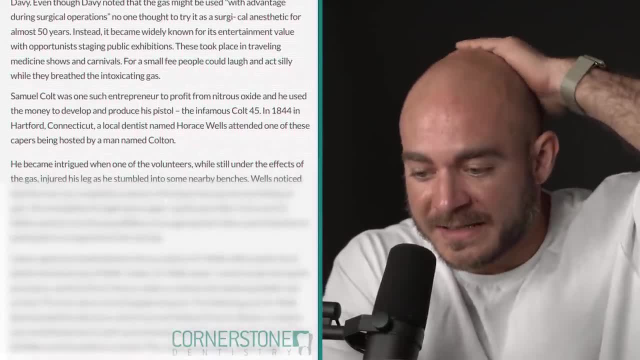 intrigued, and one of the volunteers, while still under the effects of nitrous oxide, was a medical anesthetist in Austin, Tennessee. The doctor reported that his ankle was hurting his ankle. He said that working with his ankle hurts the ankle if it doesn't fix the anus. 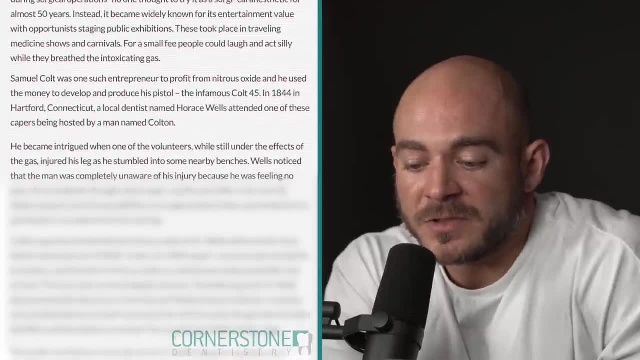 so the gas injured his leg as he stumbled into some nearby benches. Wells noticed that the man was completely unaware of his injury because he was feeling no pain. He immediately thought about applying this pain killer in his work. Dr Wells wanted to test the possibility. 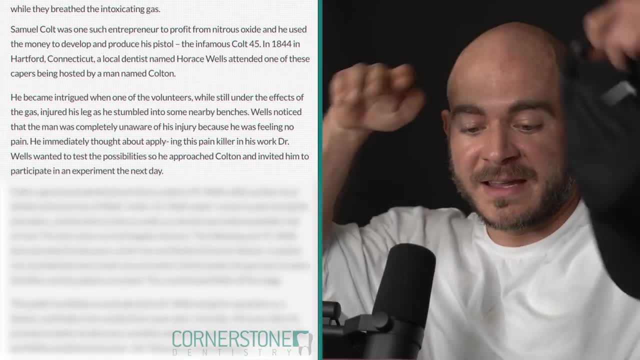 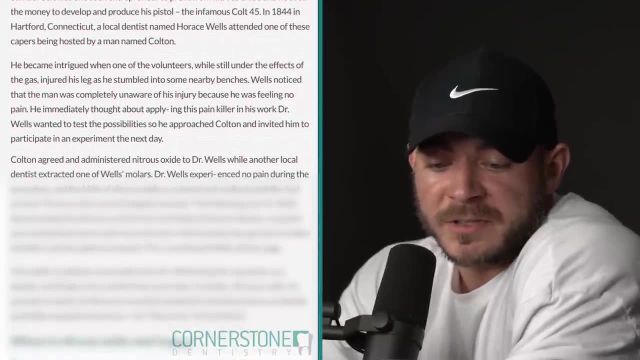 so he approached Colt and invited him to participate in an experiment. the next day, Colt agreed and administered nitrous oxide to Wells, while another local dentist extracted one of Wells' molars. Dr Wells experienced no pain during the procedure and the birth of nitrous oxide. 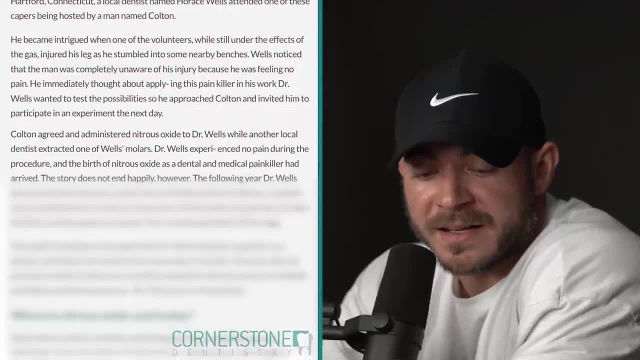 as a dental and medical pain killer had arrived. The story does not end happily. It started as a boner, but all that was lost For a few. Hopefully, however, the following year Dr Wells demonstrated his discovery at the Harvard Medical School in Boston. 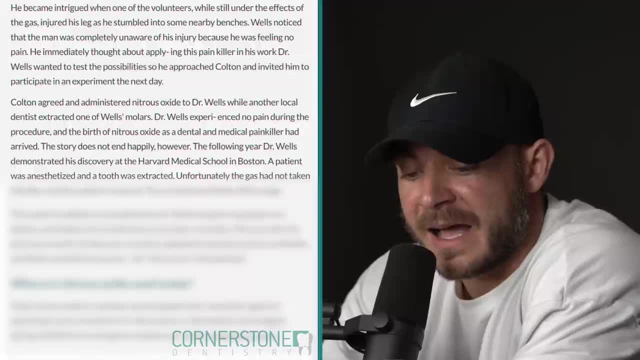 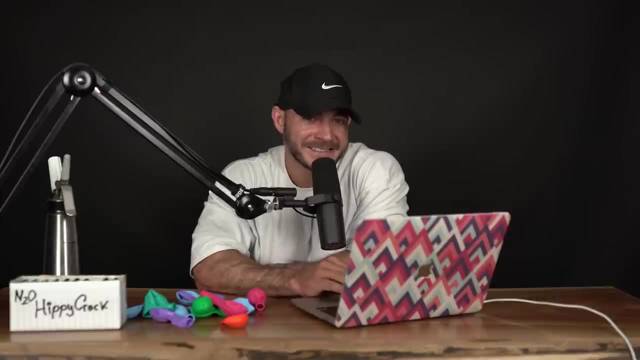 A patient was anesthetized and a tooth was extracted. Unfortunately, the gas had not taken full effect and the patient screamed. The crowd booed Wells off the stage. Got your tooth pulled out on a stage. That's wild man. 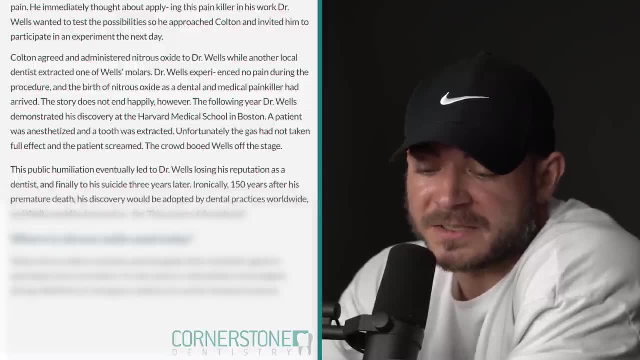 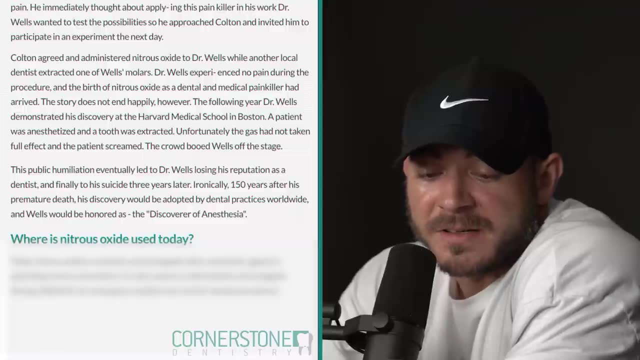 Ironically, 150 years after his premature death, his discovery would be adopted by dental practices worldwide and Wells would be honored as the discoverer of anesthesia. Wow, He discovered anesthesia. Where is nitrous oxide today? Today, nitrous oxide is routinely used alongside other anesthetic agents in operating rooms. 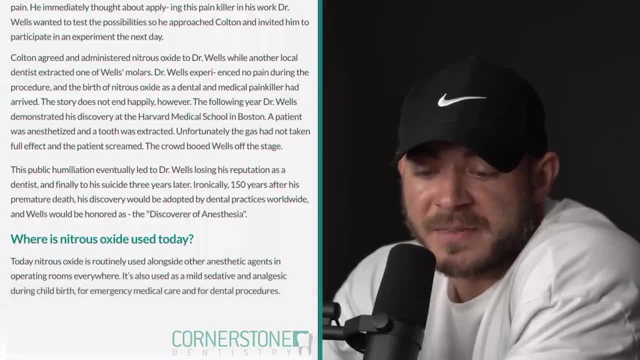 everywhere. It is also used as a mild sedative and analgesic during childbirth, for emergency medical care and for dental procedures, and for hippies who love to mix it with shit like acid and watch all the pinwheels take them to another dimension. 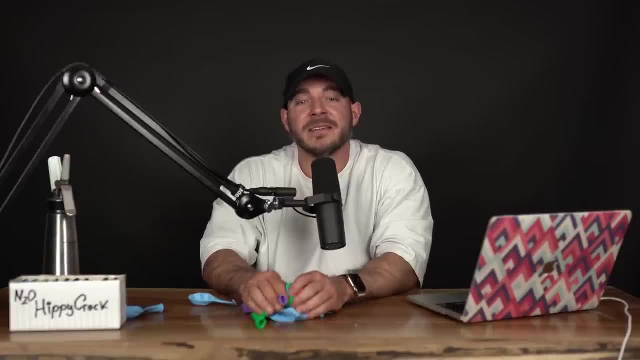 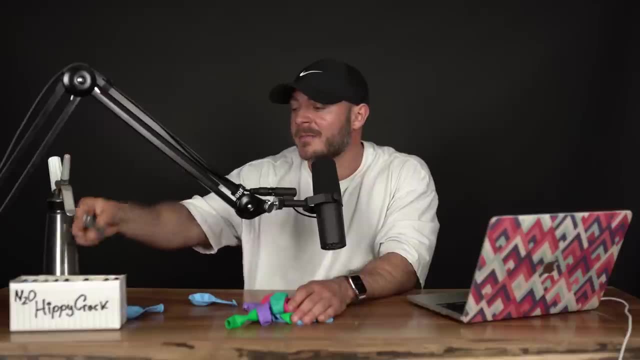 Anyway. so now you guys got the history of laughing gas. let's talk about the legality. In most places around the world this is completely legal. I mean, these are from Amazon. You can go on Amazon and buy drugs. People don't know that. 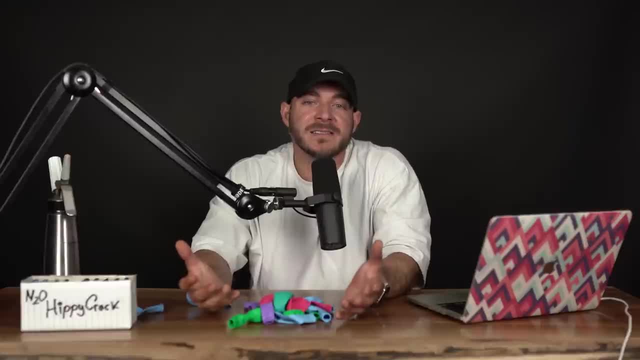 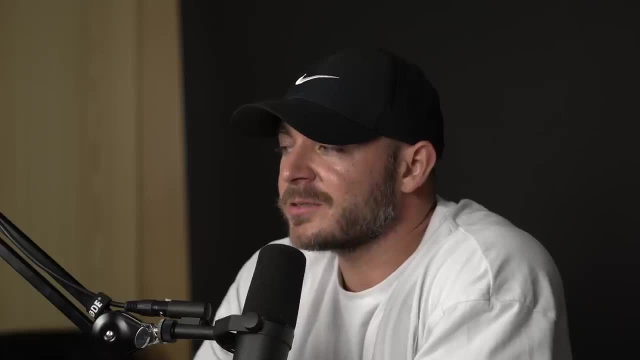 The laughing gas. you can get them in stores. You can order giant boxes, cases of fast food, Thousands of them, If you really wanted to price ranges depending on where you live. Now let's talk about the danger. Now they're generally safe, but there is an issue with B12.. 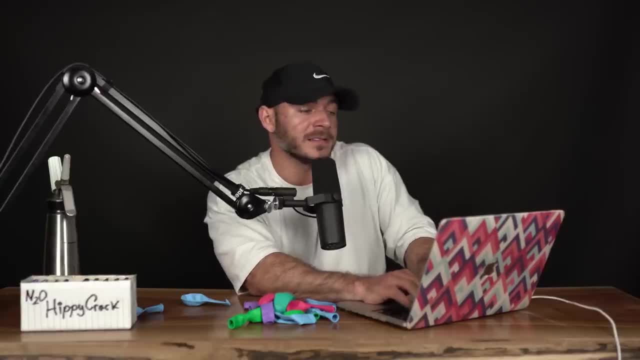 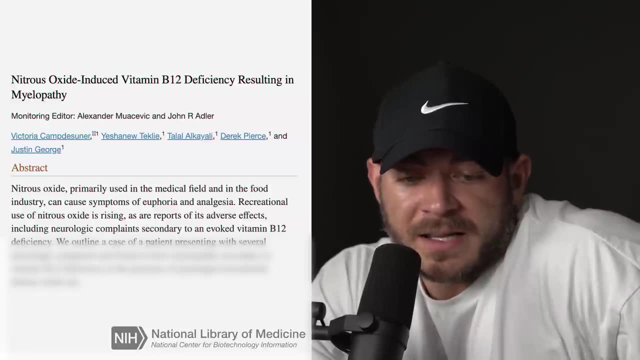 Let's look it up So I don't explain it wrong. Basically, if you take laughing gas all day, every day, you will get a B12 deficiency which could actually be fatal Nitrous oxide induced vitamin B12 deficiency. We outline a case of a patient presenting with several neurological symptoms and found. 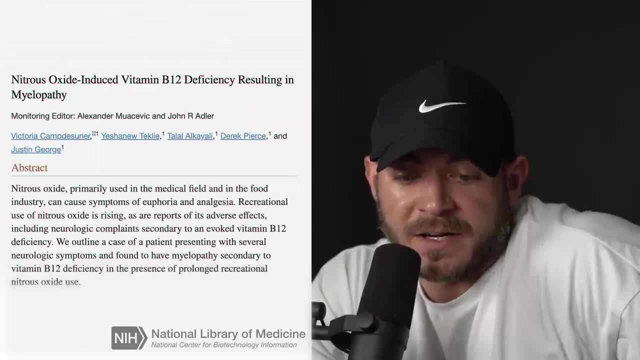 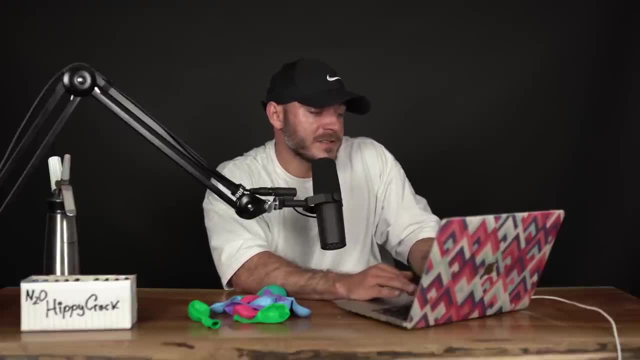 to have myelopathy secondary to vitamin B12 deficiency in the presence of prolonged recreational use of nitrous oxide, Die From B12. So a vitamin B12 deficiency, a deficiency in the production of red blood cells due to a lack of vitamin B12, can cause permanent neurological damage that can lead to death. 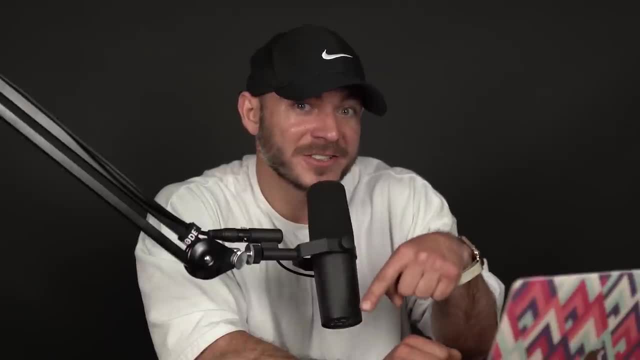 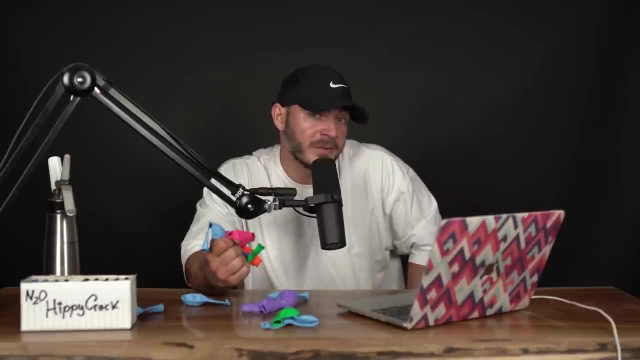 if it's untreated, Not totally safe. You hear that Permanent neurological damage. If you're doing tons of them, be careful. So, basically, if you're going to use this stuff, you need to take vitamin B12 or just use it sparingly, because it only lasts- like I don't know- 30 seconds. 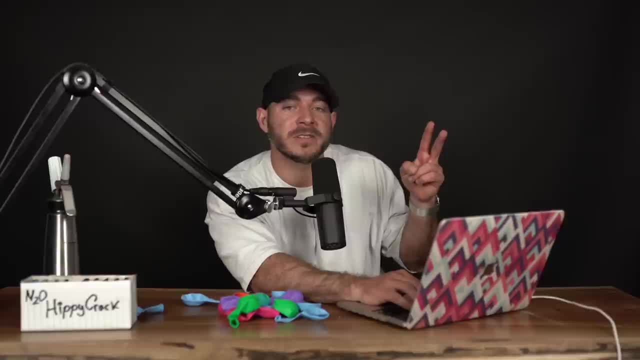 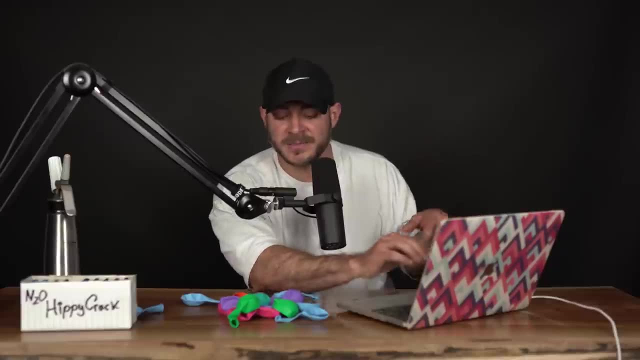 It's not very strong And there's two ways to administer it, which we're going to explain. There's the drug addict way and then there's the safe way. Of course, I advise everyone to the safe way, but before we get to that, I need to make 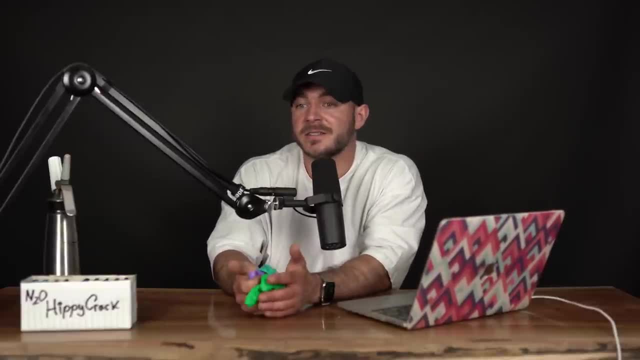 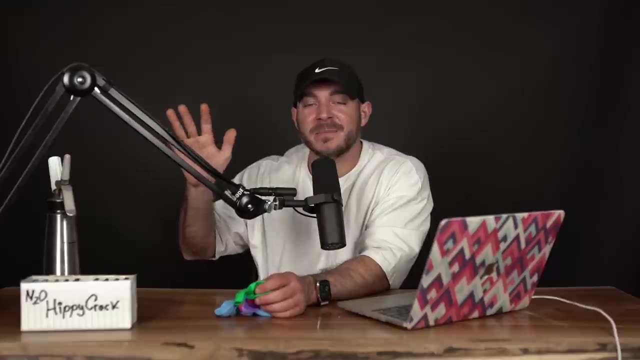 it clear that, even though this is a legal substance, you know used in the medical system, used in food, anyone can buy it. This video is not made to promote the use of it. Any substance can be dangerous depending on the intent behind it. 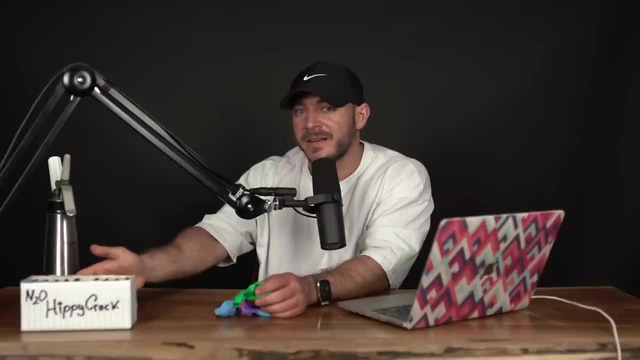 You could just be sitting in your basement doing balloons all day. I've been there, And when it gets to that point, yeah, I would say it's dangerous on a well, just emotional level. You can use it to run away from your problems. 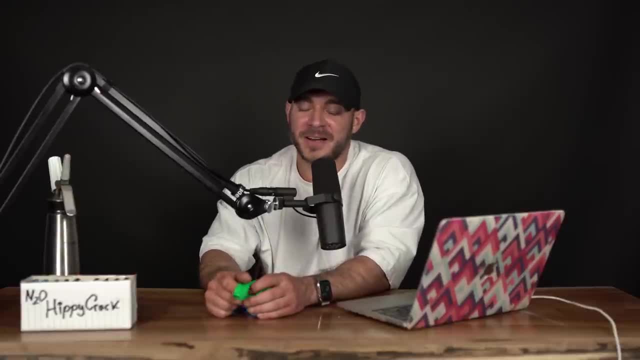 It's just like any drug. It's not going to be as strong as something like heroin, of course, but it does offer a very short, quick escape. And when mixed- which is the highlight of this video- when it's mixed, that's when it's. 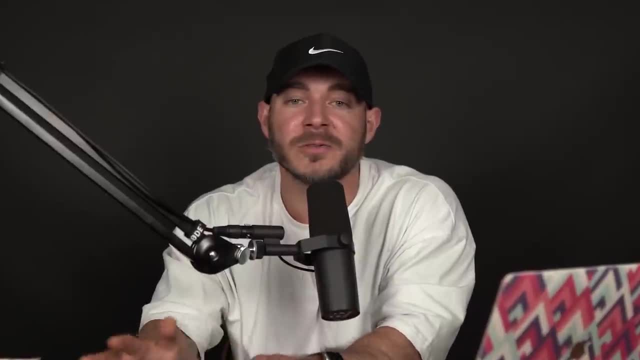 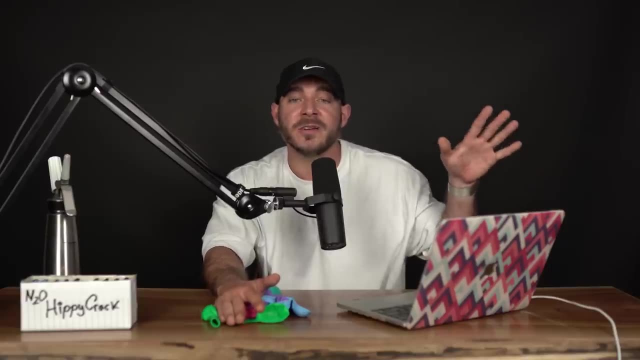 true potential really shines. But just to be clear, we are not making this to promote or glorify the use of any compound. We're making this for education, to educate you guys about the history of it and to show you, if you're going to do it, how to do so safely, so you don't hurt yourself. 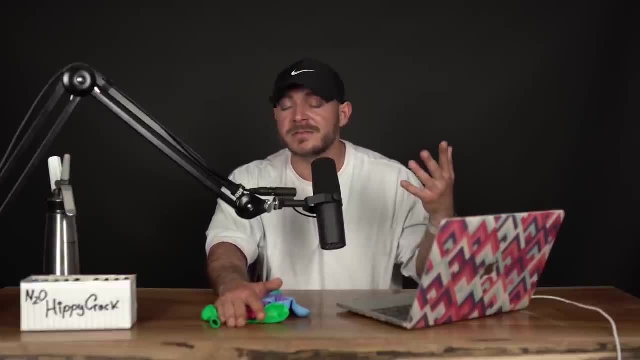 Of course, the best form of harm reduction is always going to be abstinence, So just don't do this stuff. But if you're going to, let's at least get this taboo out of there so I can show you how to do it safe. 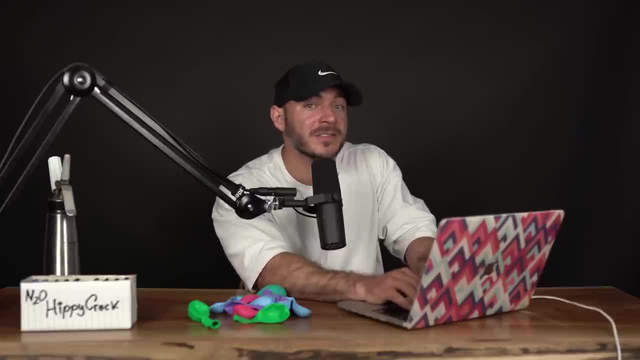 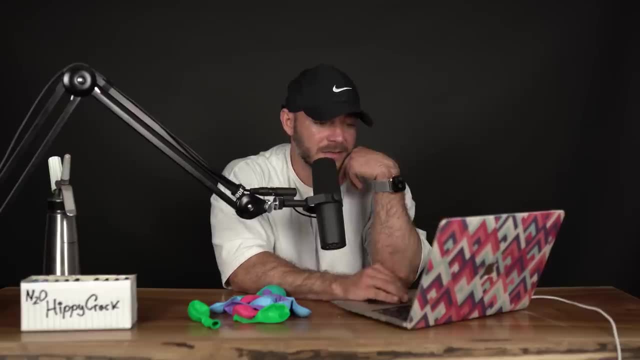 Now, what constitute tons? Is it 20 balloons, 50 balloons, a thousand balloons in a sitting? I have no idea. Everyone's mileage will vary. Depends on your own constitution, right? So let's see here. So dosage is basically half to one full cartridge. 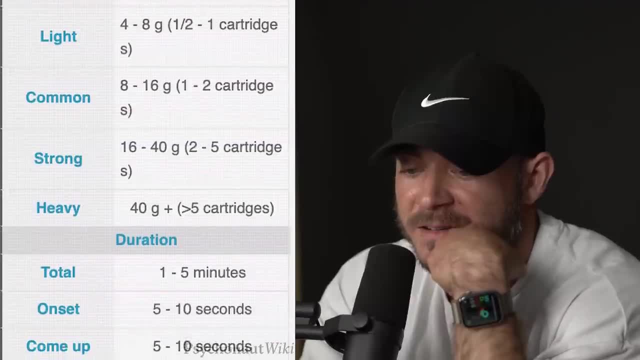 Common people take one to two cartridges at last. total one to five minutes. onset: five to 10 seconds. Yeah, it's pretty instant Peak: 15 to 30 seconds and offset one to five minutes. After effects: 15 to 30.. So what I find the after effects are is you generally feel very relaxed, like it could be a great sleep aid. Again, don't recommend it, but if you're like in a pinch, it's probably safer than benzodiazepines. 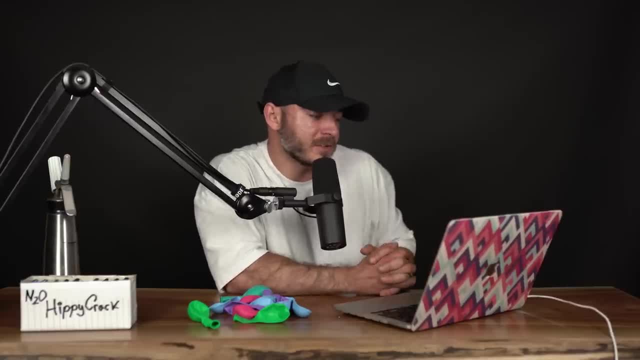 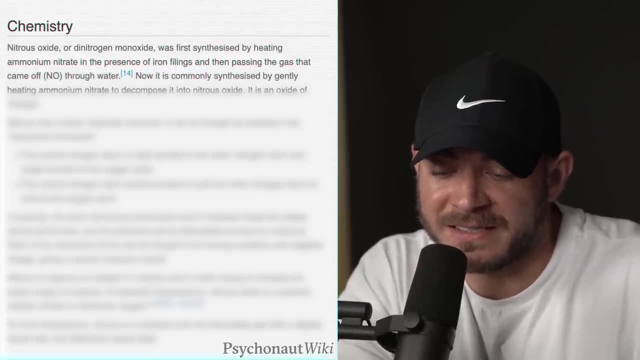 Actually, I know it's safer. And let's look at the chemistry. This is very interesting too. Nitrous oxide, or dinitrogen monoxide, is completely synthesized by gently heating ammonium nitrate to decompose it into nitrous oxide. Nitrous has a linear molecule structure. 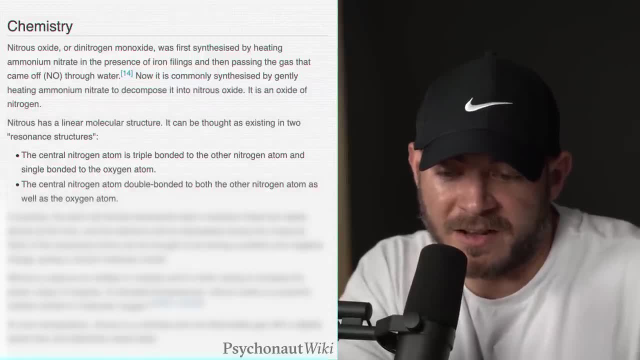 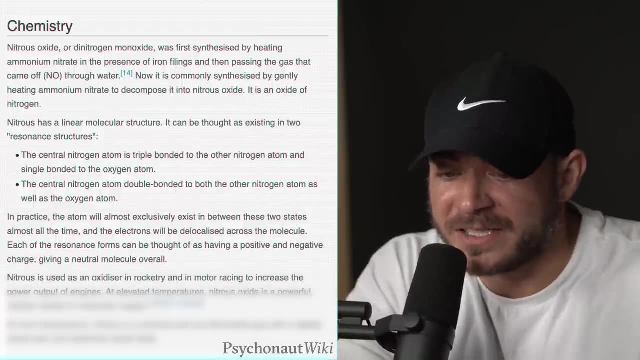 The central nitrogen atom, double bonded to both the other nitrogen atom as well as the oxygen atom, And here's a picture of the molecule. Nitrous is used as an oxidizer in rocketry and in motor racing to increase the power of engines. Nitrous oxide is a colorless, nonflammable gas with a slightly sweet odor and distinctive. 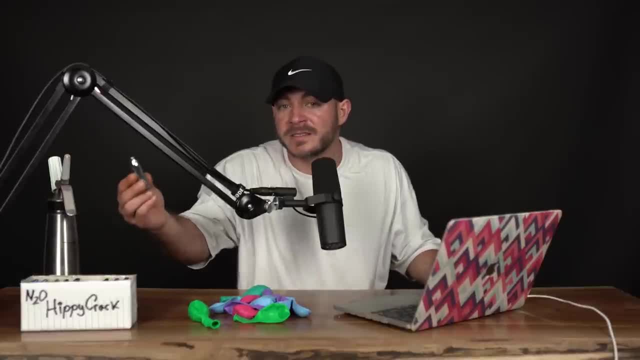 sweet taste. Now you'll know if you have good balloons, because the good ones you'll actually taste a sweet taste. The bad ones you won't. We're going to get into why you use a balloon in a minute. Now let's talk about pharmacology. 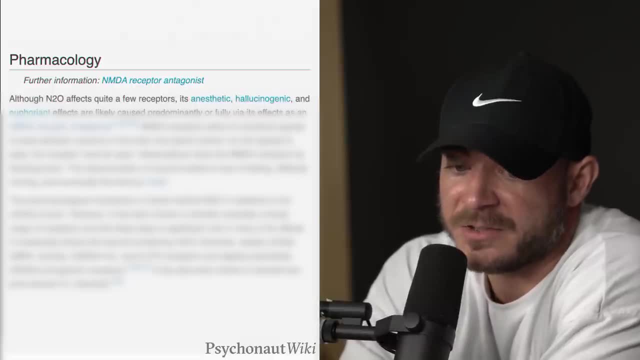 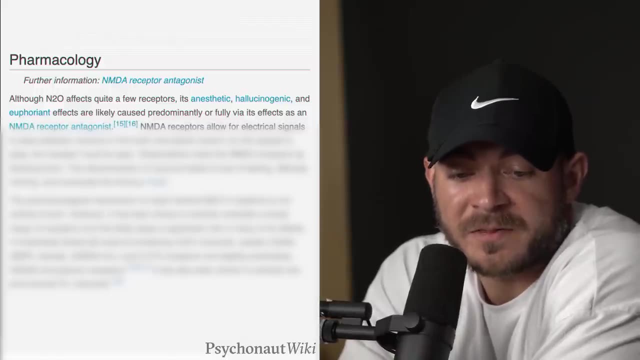 Although N2O affects quite a few receptors, it's anesthetic. hallucinogen and euphorian effects are likely caused predominantly or fully via its effects as an NMDA receptor agonist. You might remember that name from things like ketamine. they are actually both dissociative. 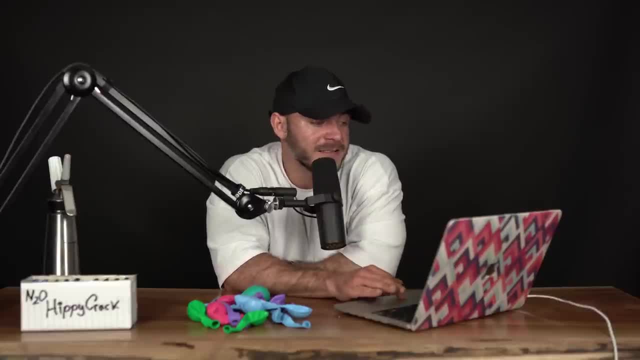 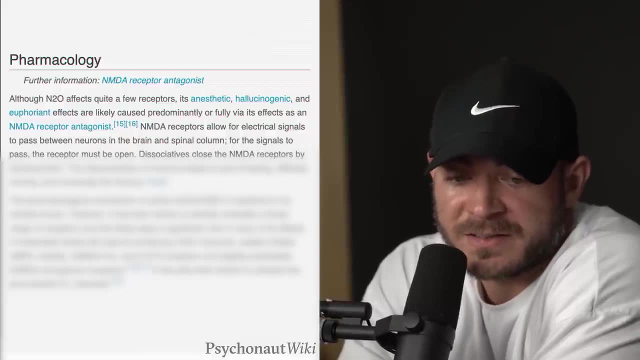 compounds, Same with stuff like PCP. these are all in the dissociative class. NMDA receptors allow for electrical signals to pass between neurons in the brain and spinal column. For the signal to pass, the receptor must be open. Dissociatives close the NMDA receptors by blocking them. 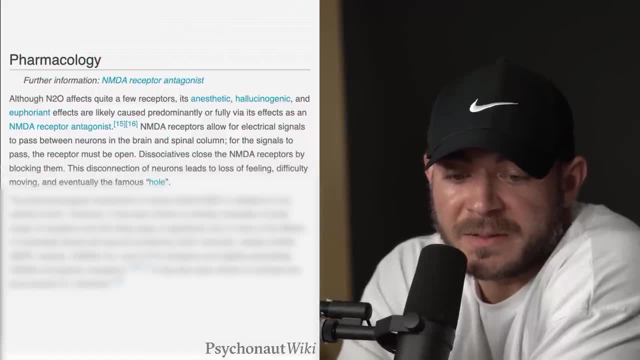 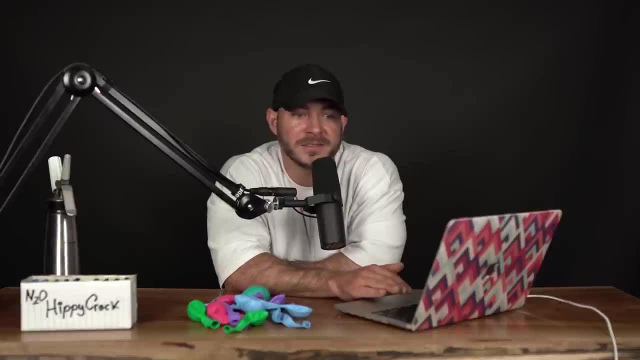 The disconnection of neurons leads to loss of feeling, difficulty moving and even the famous hole. You're not going to K-hole on this stuff, but you can pass out. I've done it very easily- And then, if you're standing you will fall, so you need to be seated. 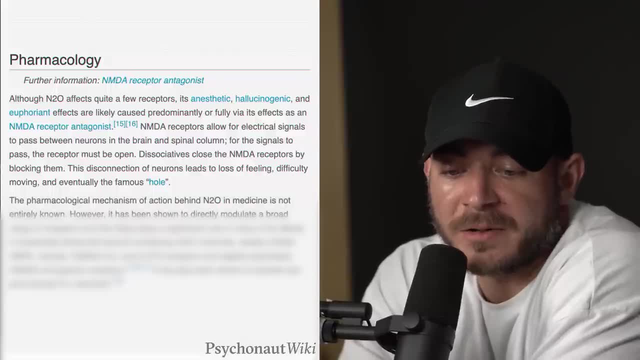 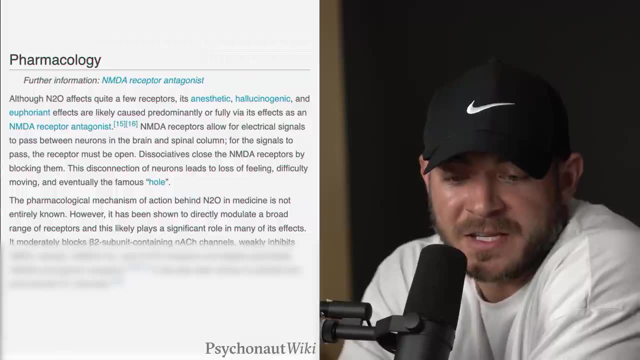 The pharmacological mechanism of action. The reason behind N2O in medicine is not entirely known. however, it has been shown to directly modulate a broad range of receptors and this likely plays a significant role in many of its effects. It moderately blocks B2 subunit containing NACH channels weakly, inhibits AMPA KNAIT. 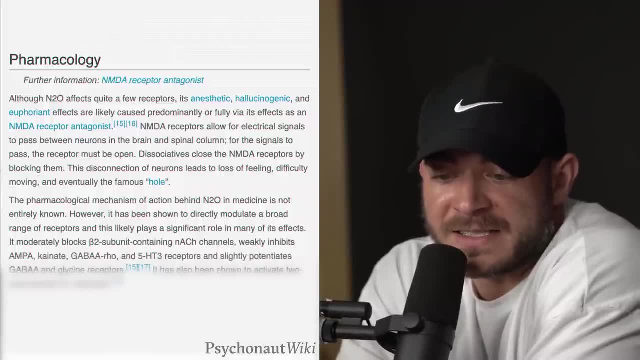 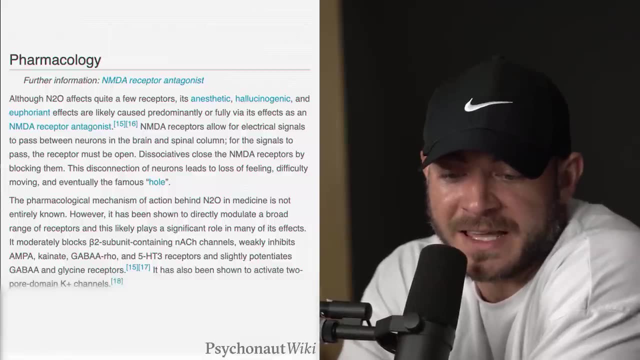 GABAA, RHO and 5-HT3 receptor and slightly potentiates GABA and glycine receptors. It has also been shown to activate two pore dominant K-plus channels and some people speculate that it actually has some effect on the opioid receptor. So let's get into it. It's not proven, but some people do think that because they found, when they were in their withdrawals, say, of heroin, this temporarily alleviated withdrawal symptom for, I don't know, 5,, 10 minutes. 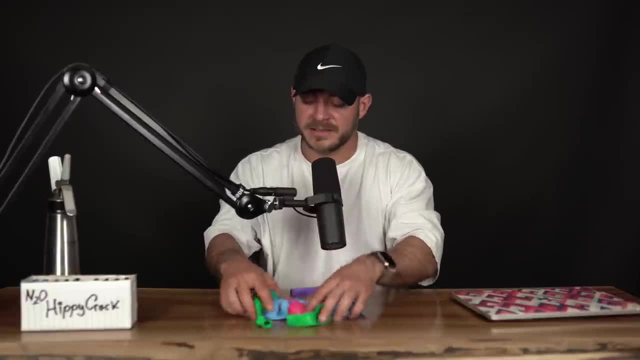 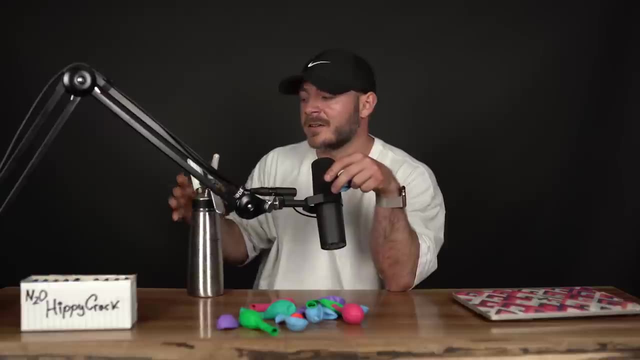 Now that we've got all the data out of the way, let's explain basically how people take this. So the reason why you use a balloon- and this is a legit whipped cream dispenser- you can actually get things called crackers. They're very little and they're designed just for doing this, but I like doing it this way. 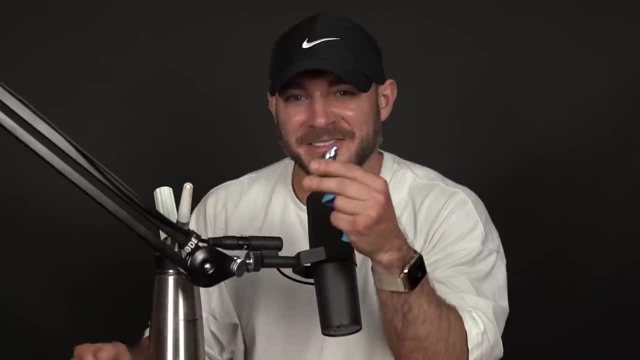 The reason you use the balloon is because this is compressed gas and it's cold. You'll notice As soon as you do it here, I'll show you. and this one's not going to be cold. You have to pull it out right away. 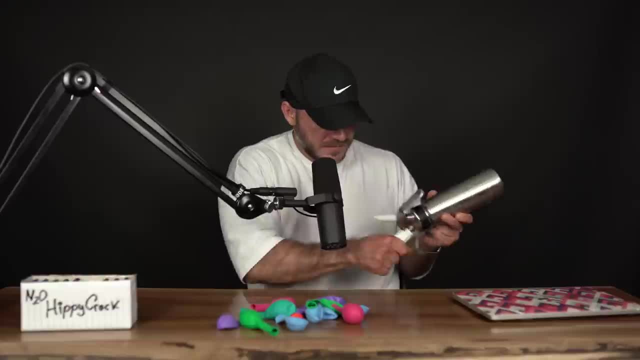 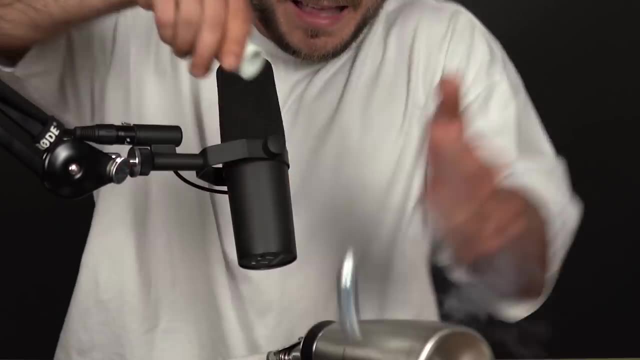 That's what she said. So watch this. You'll be able to see how cold it is. Okay, Got to be fast. Ooh, lost some there. See it smoking? Whoa, look at that. And it burned me. 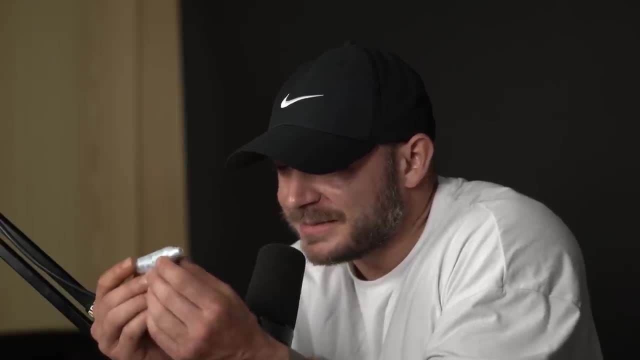 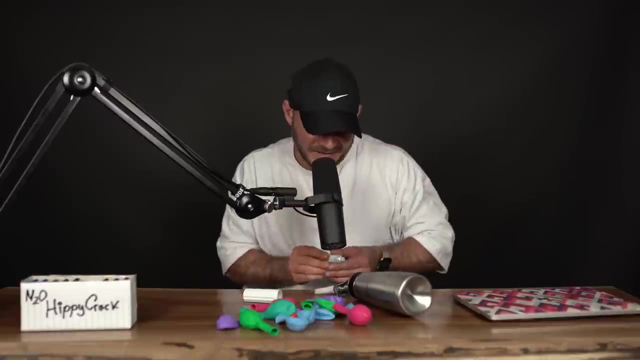 That is, ooh, it's ice. Look at that. Wow, Put it near my face because I'm very hot right now down here, Holy crap. So you use the balloon, because if you were to say, just do that and then put this to your, 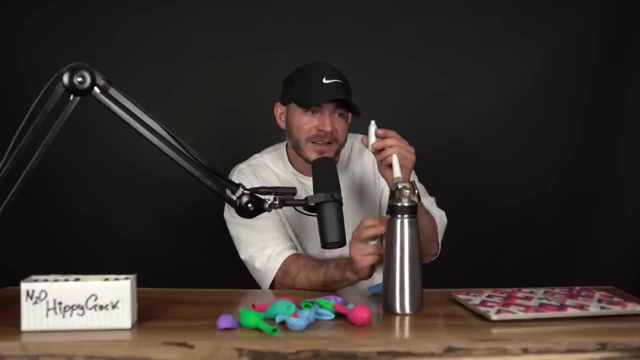 remote- this is the harm reduction part of the video- and suck in. what do you think that's going to do to your lungs? You think that's going to be comfortable? Now, I don't think your lungs have feeling receptors, but you don't want to damage them. 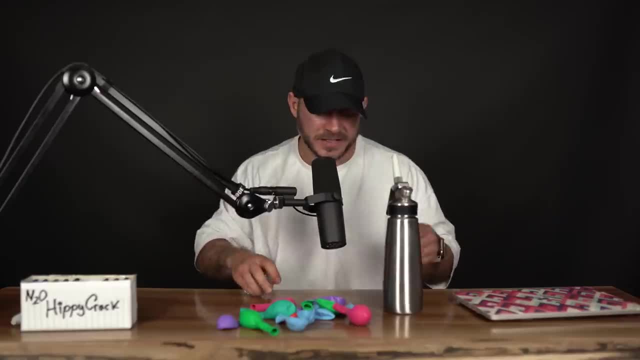 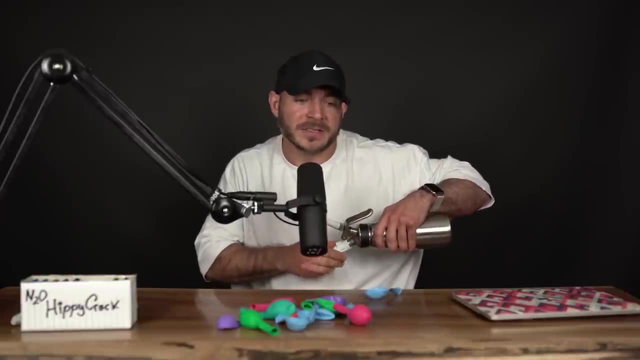 with fucking freezing cold gas. So, yeah, this is why you do it this way, And now we're going to explain the effects on their own. Now, on their own. and what it really feels like is: you get a buzzing in your ears, You hear a noise, You start seeing these slight pinwheels. With higher doses the pinwheels get more predominant and they spin all around and you feel a little wonky. Some people giggle, I don't giggle. You feel like a slight mood boost, like all of a sudden you just feel a little bit better. 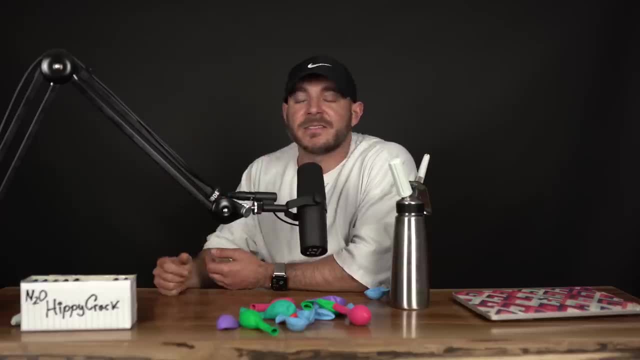 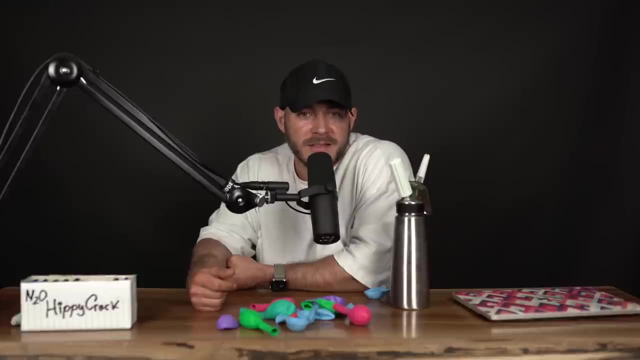 more comfortable If you're going through some trauma. all of a sudden it lessens and you're like, oh, this is easier to handle. It makes life just a little bit easier to handle. But by no means is this a very intense drug and it's very short lived. That's why people just do them one after the other, after the other, because the effects when you get a tolerance it feels like 30 seconds to a minute. The tolerance makes it last nilch, It's just like so short. 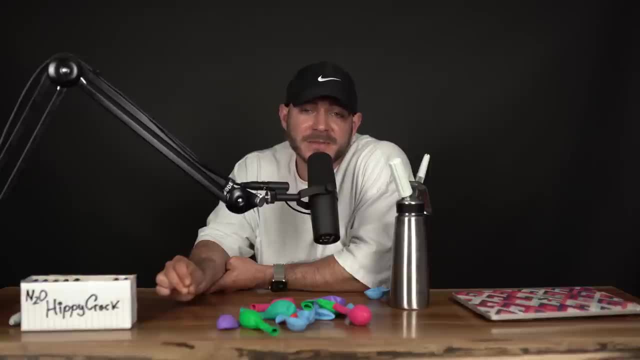 And if you're after just some relief, You got to just keep doing them. So it's pretty freaking time consuming. But where it shines actually is when mixed, So depending on the compound you mix it with, I call it. it's like psychedelic tofu, because 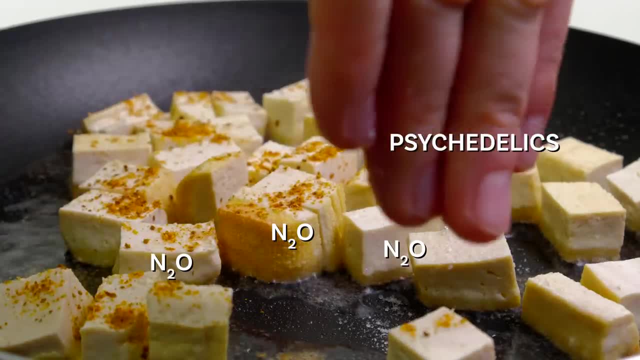 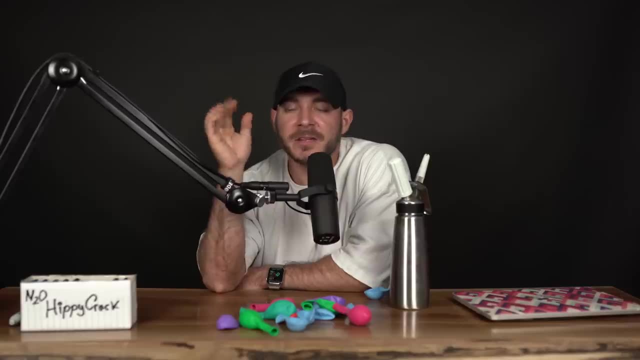 tofu doesn't have a flavor until you add the spices to it. So the drugs of the psychedelics are like the spices. Now on something like LSD, I have a lot of experience mixing those again. Don't advise this. The pinwheels that you see- they start to zoom out almost. 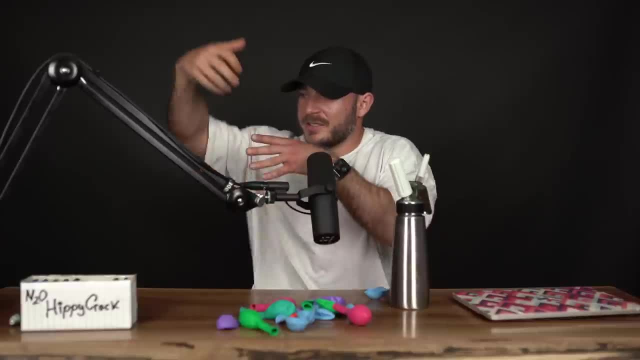 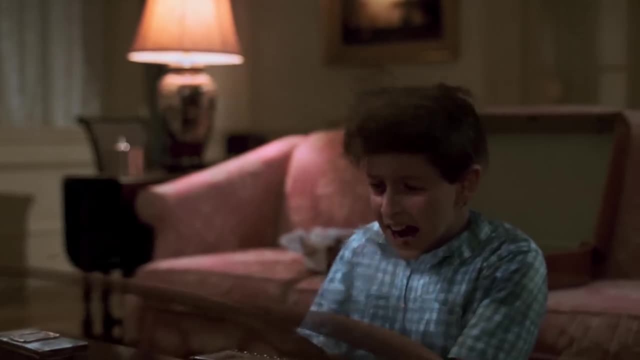 And your body. I've I've watched like like picture, like I'm stretching really high, Like um picture, like a black hole where the body's like stretching unusually, like into it, Like all of a sudden he becomes like 200 feet tall and he's like you know, it's just that. 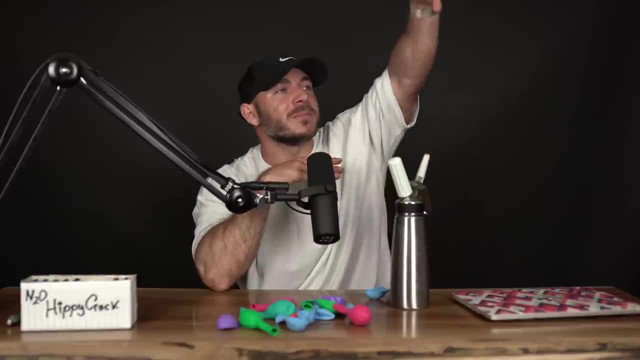 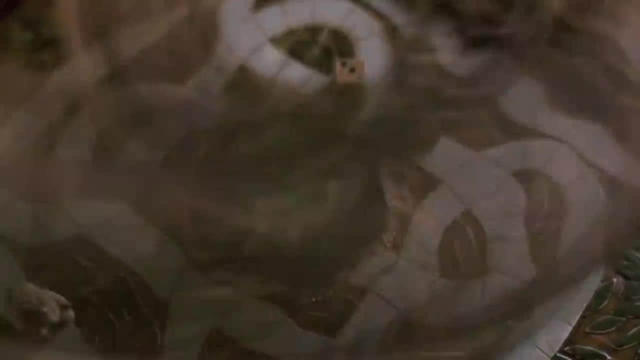 image of someone stretching. I can see that. I can see my whole body stretching up into what looks like a point on the horizon And then, as my body's stretching, it starts spinning and twirling into its own pinwheel And I get like sucked out. 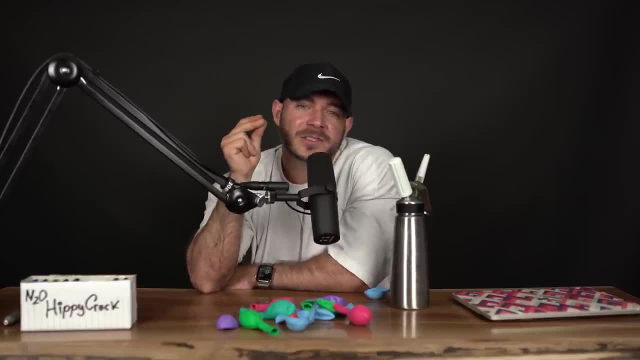 On acid. doing this feels like a very light version of DMT. It's like DMT light because you get sucked out of your body, But the difference is you're not going to a new dimension. It's like a very light version of DMT. 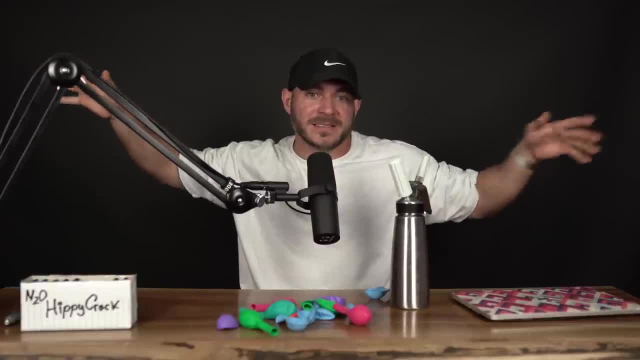 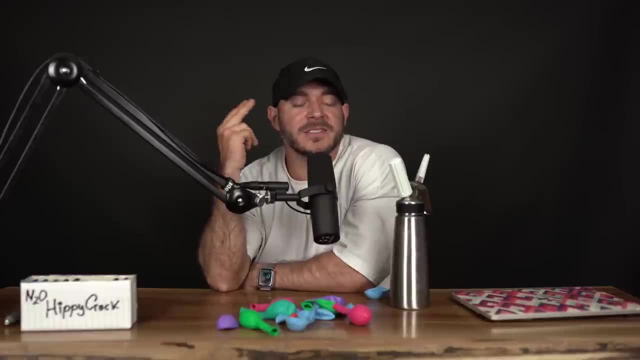 It's almost like you're just in some kind of a void, And then in that space, this is again. this is mixing with a good dose of acid. When I'm sucked out, I'm always in a loop, So, whatever, the last thing that I saw, was it just loop. 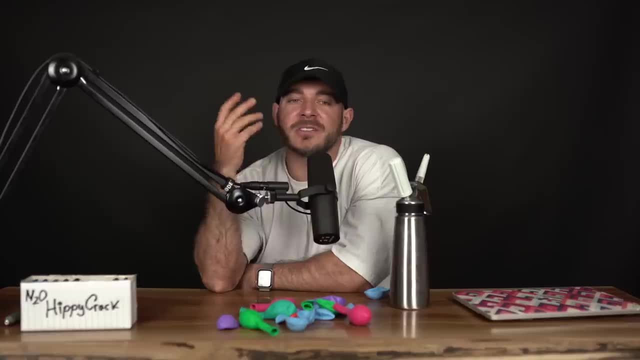 So if it was somebody saying to me like, Oh my God, that's crazy, I would just hear: Oh my God, that's crazy, Oh my God. And it would be like a loop. but it would sometimes be like it's pitch black by the. 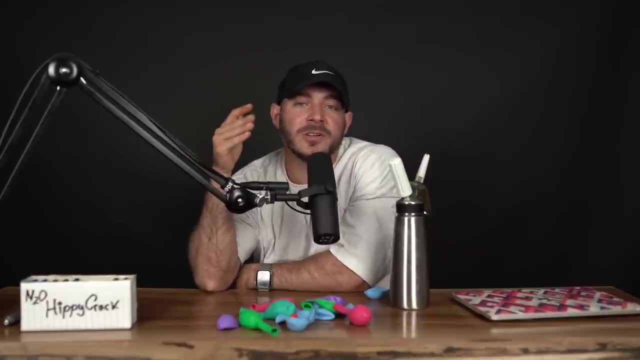 way when you're in this and it just keeps like repeating and repeating and you have no control over this repetitive feeling, And it can feel more than just an audio. It can feel like You're actually reliving that experience over and, over and over again, to the point. 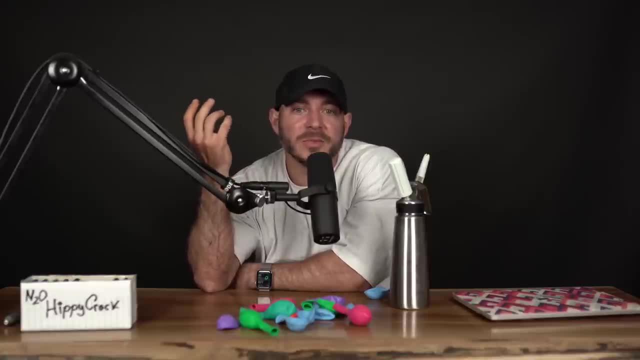 where you get scared and you're like, Oh my God, when is this going to end? It's like an infinite loop And when you're in it it feels infinite. And then when you come back, I've come back and I've been like, Oh my God, that was terrifying. 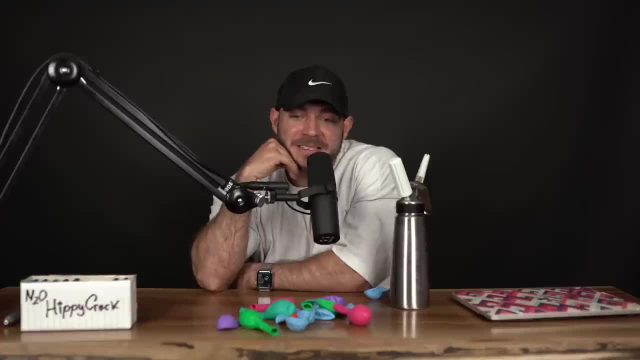 I'm never freaking doing that again Now. I've also mixed it with DMT, which most people will never do And it's probably not advised, And it felt like it was relocating my consciousness. Now, keep in mind this isn't on breakthrough doses, just on like average, maybe threshold. 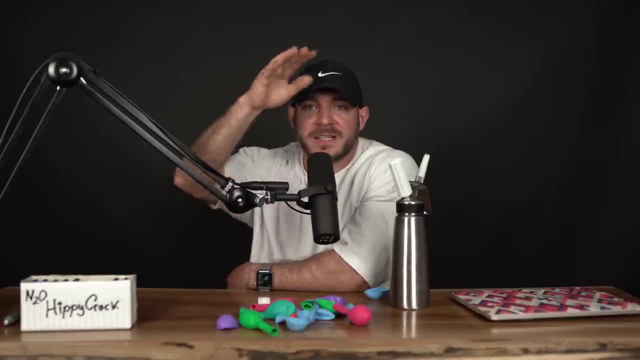 maybe go in the waiting room. doses felt like my consciousness was getting Transferred to different parts of the room, Like I was Spider-Man, almost like I was in the corner of the room looking back at my body And then, before I could tell, like, Oh my God, I'd like become a cup. 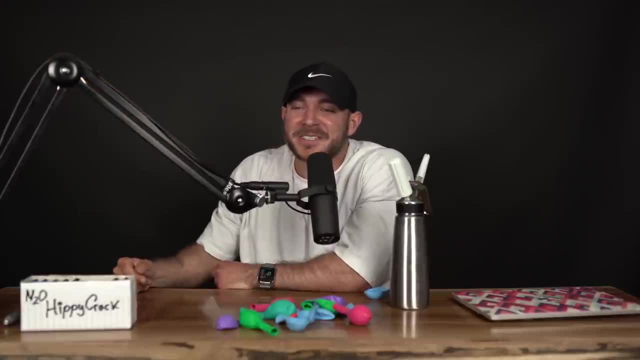 That's what it did. I became inanimate objects now on things like MDMA, which most people have their experience mixing it. The first time I did it it felt like I was going up up, you know, on a roller coaster and then woo down. 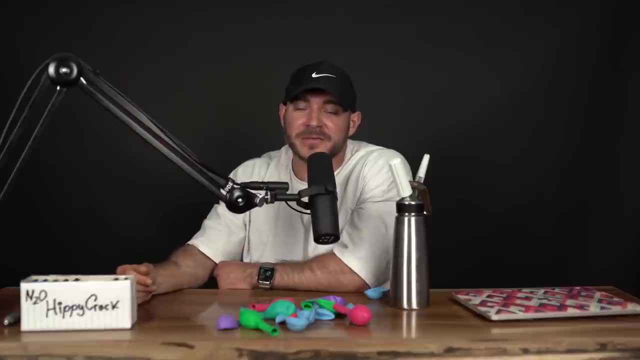 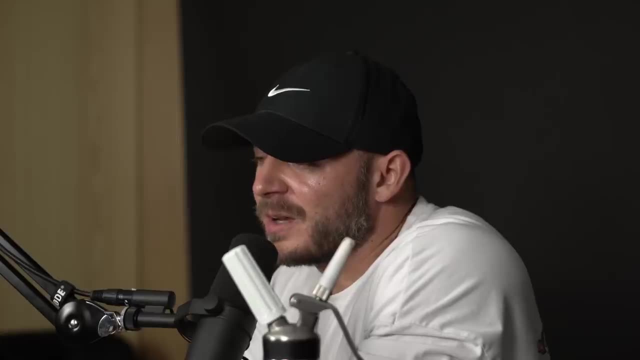 It was a roller coaster feeling. really, it just accentuates whatever euphoria or pleasure you're feeling on things like MDMA. Now some people are crazy and they mix dissociative with dissociative. they do it with ketamine, which I can't really say. I can't really speak on. I've tried that once in the past and I just don't remember. So leave your replies below on what that was like. I've also tried it on several research chemicals. It's generally going to be one of these things. 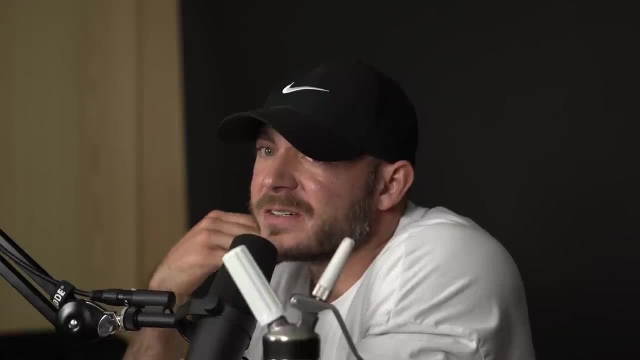 I have not tried it on no, I've tried it on mushrooms. I think mushrooms was actually very similar to LSD. But anyway, now that we've got the effects of the way, let's show how people you know how you're supposed to do it. 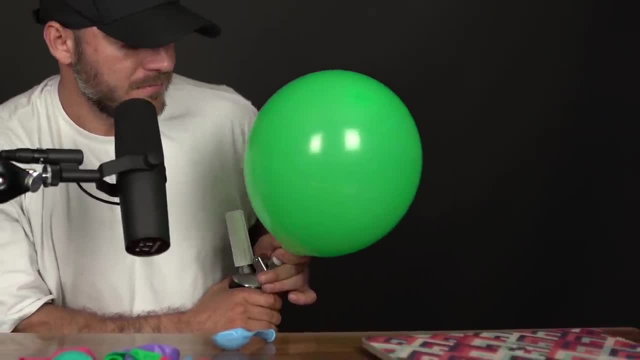 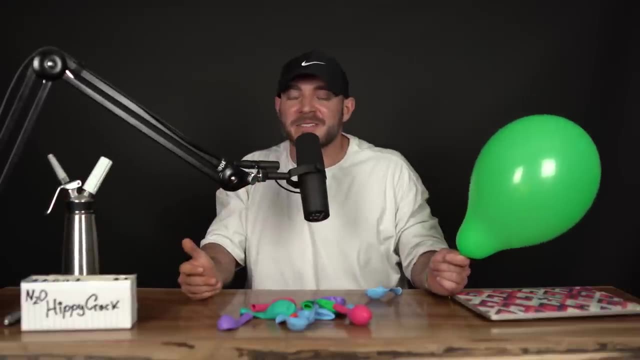 And unfortunately, okay, there's fucking two in here. That's way too much. This is huge. They're usually half this size. Unfortunately, we can't show any Consumption even of a legal whipped cream thing on YouTube, So if you want to see that scene, you have to join our Patreon. 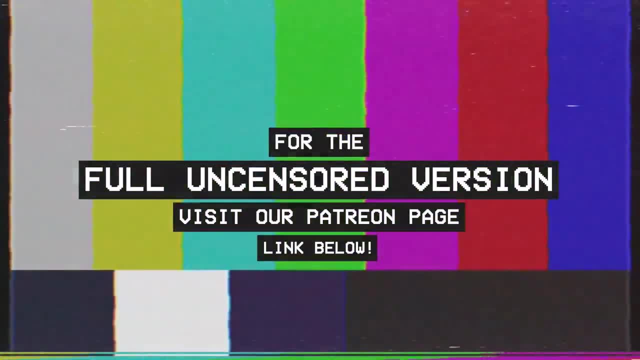 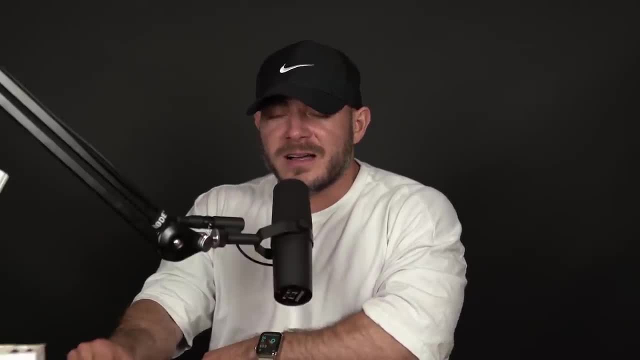 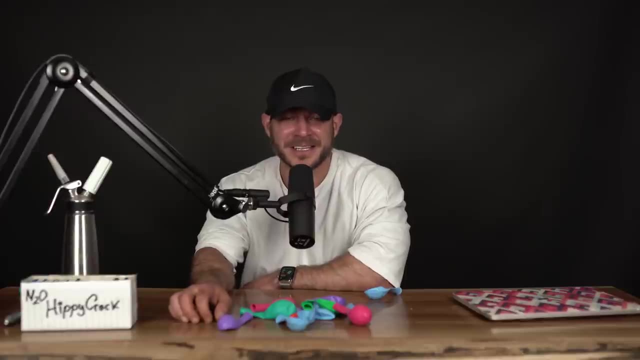 We're just going to skip past that anyway, Now that we have done the effects portion. yeah, now you guys know all about the safety of nitrous, you know. but the history of nitrous you know, with the V12 deficiency, you know. 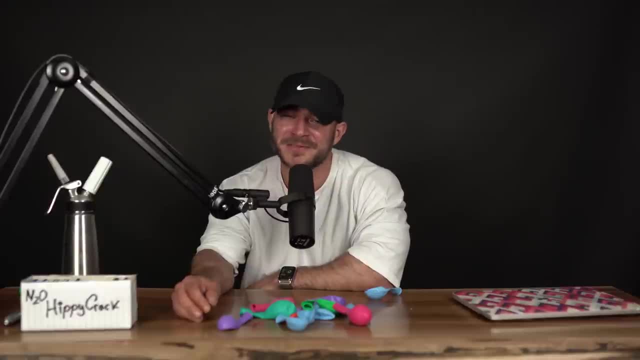 but everything. Now you guys got all the points, So that's the end of this video. If you enjoyed this video, make sure you leave it with a big thumbs up. And again, if you want to see the uncut version, head on over to our Patreon page, head on. 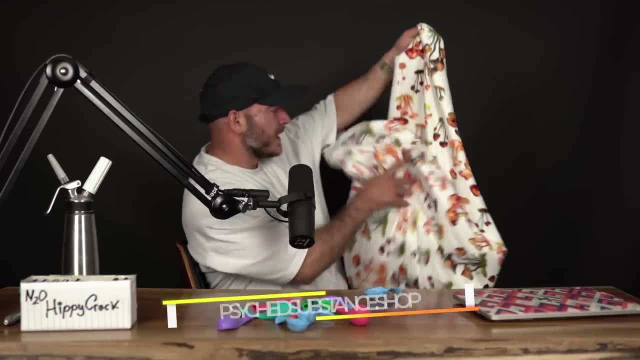 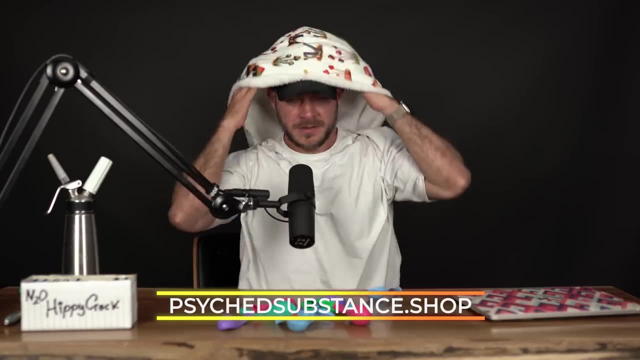 over to psychsubstanceshop to pick up your very own food and trip blanket These things. we've been waiting for ages for the white ones and they should be delivered soon. So if you ordered a white one, it's coming soon, Yeah. 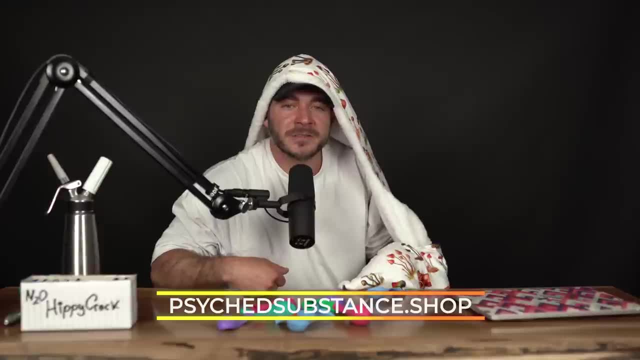 These are super soft, made by trippers for trippers. You got the pockets. This is to wear on you where, where, while you are having a super intense psychedelic trip. So head on over to psychsubstanceshop to pick one of those up and, yeah, leave it on. 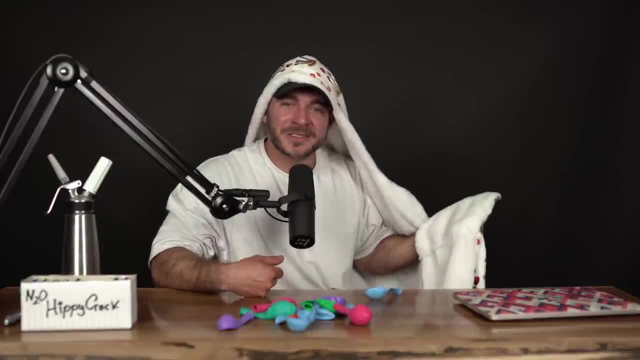 your own. And, yeah, leave a comment for the algorithm and let me know if you enjoyed this video. I will see you guys all in the next one. Cheers. 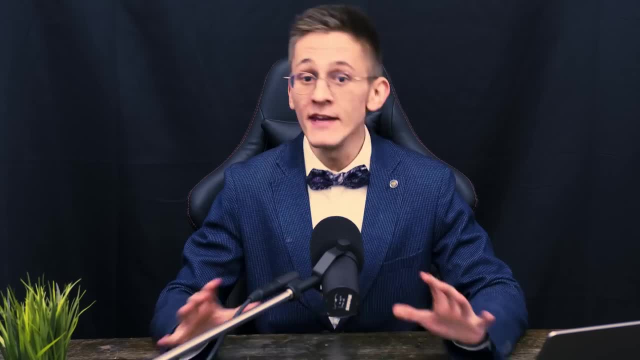 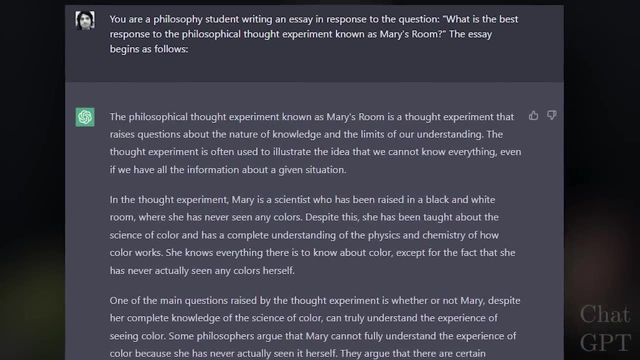 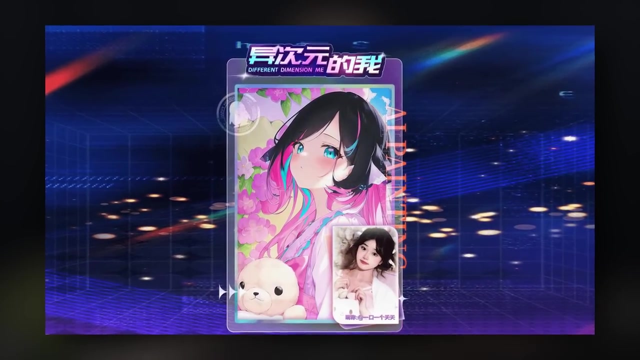 The year 2022,, which has recently passed, can easily be called the year of neural networks. After all, we got a language model which can write you a surprisingly decent essay, an AI art generator and even a platform which turns any image into anime.